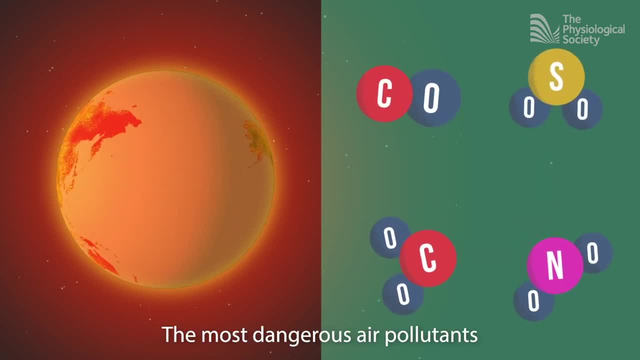 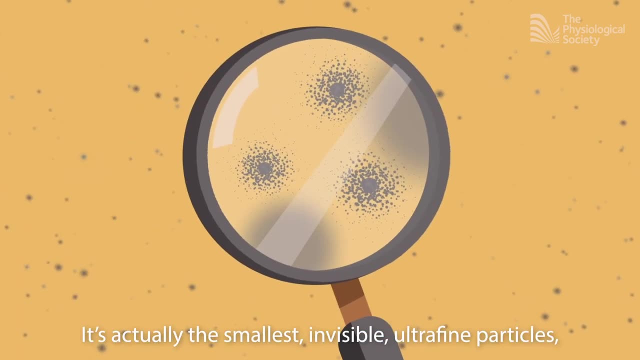 pollutants in the air that have harmful effects on the body. The most dangerous air pollutants for our health are particles. Particles can be made of different substances and have different sizes. It's actually the smallest. In this case, it's the smallest. 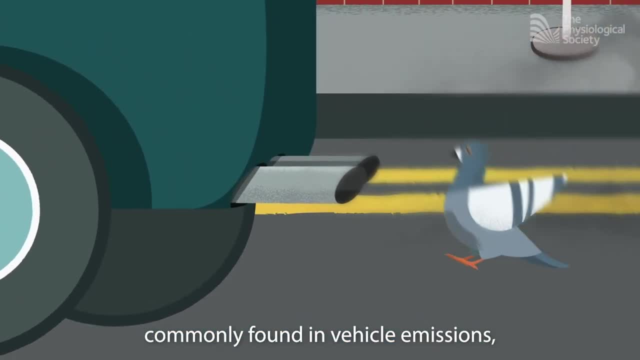 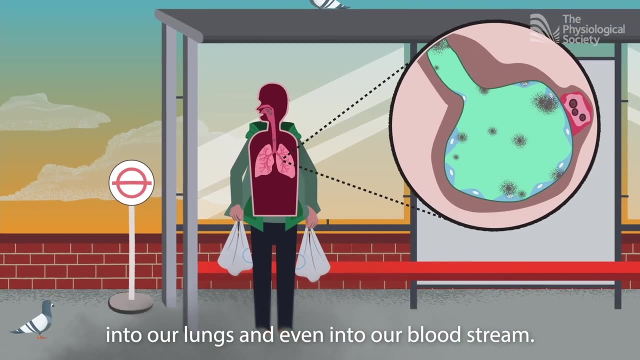 visible ultra-fine particles, commonly found in vehicle emissions, that are the most harmful. These particles are small enough to travel deep into our lungs and even into our bloodstream. There they play havoc with the cardiovascular system, changing the rhythm of the heart. 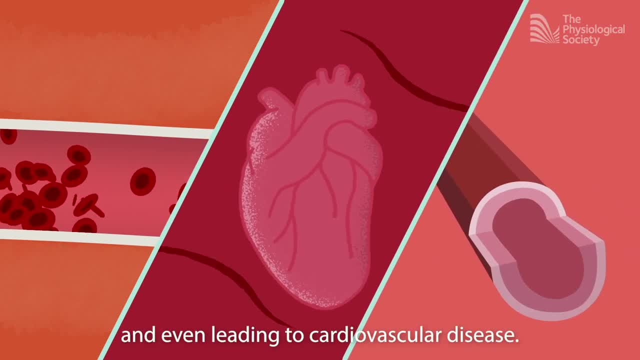 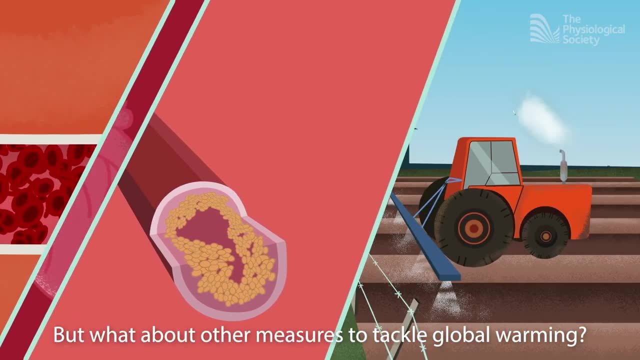 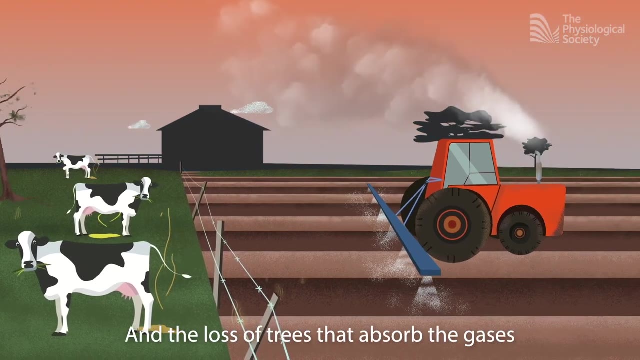 thickening the blood, making arteries more stiff and even leading to cardiovascular disease. So reducing emissions will improve the health of the planet and us. But what about other measures to tackle global warming? Our dietary demands also produce air pollution from agriculture and the loss of trees that absorb the gases that cause global warming. 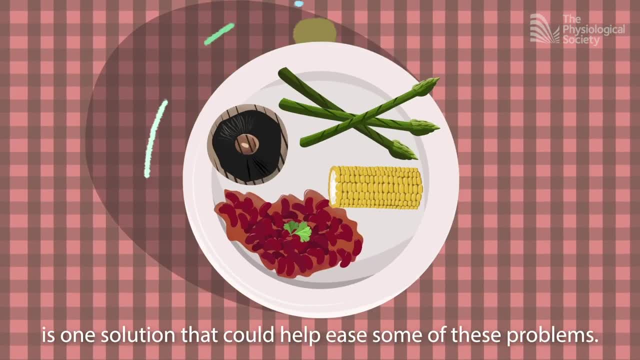 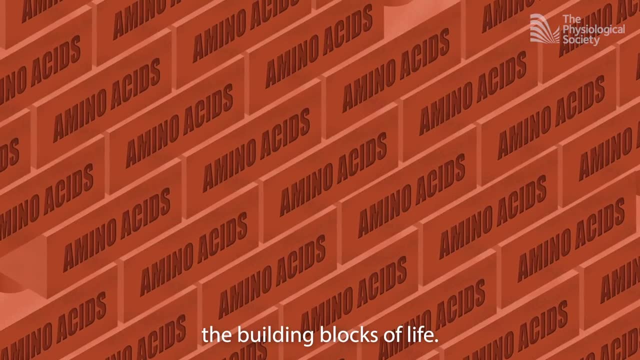 So moving from a meat to a more plant-based diet is one solution that could help ease some of these problems. The challenge is that plant-based proteins can lack some essential amino acids- the building blocks of life. We need these amino acids to build muscle protein. 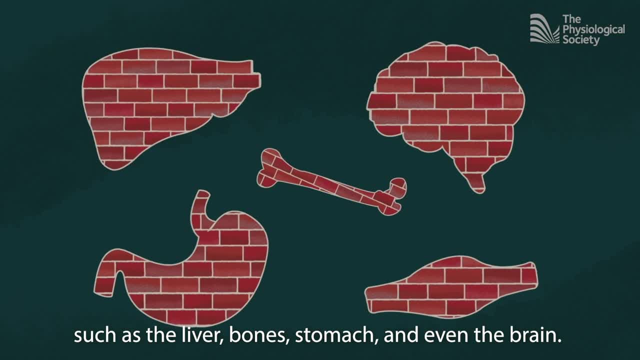 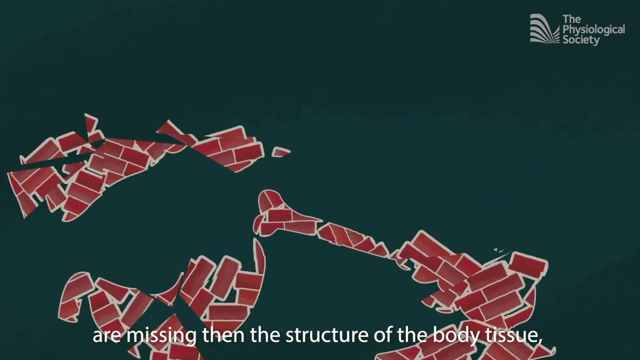 as well as other crucial body tissues such as the liver, bones, stomach and even the brain, And, like bricks in a wall, if certain amino acids are missing, then the structure of the body tissue, including muscle, will be weaker. 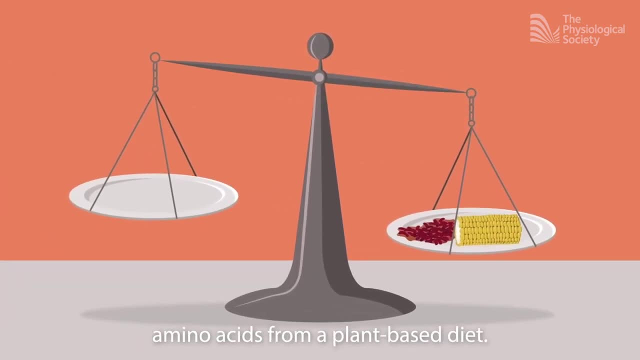 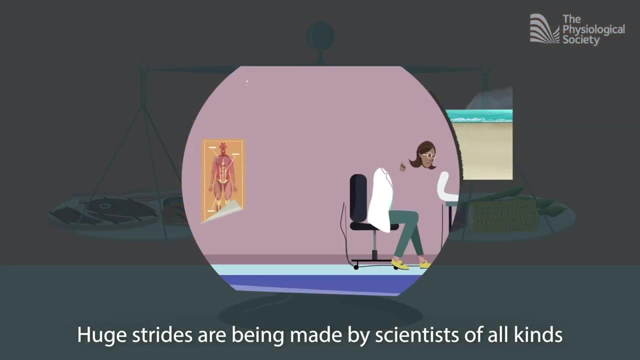 That's not to say that we can't get the required amino acids from a plant-based diet, but a carefully considered and balanced diet will be needed to prevent muscle loss and reduce climate change. Huge strides are being made by scientists of all kinds to assess the effect that climate change will likely have on our lives. 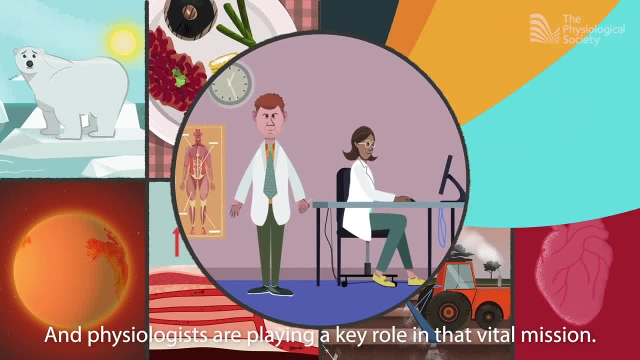 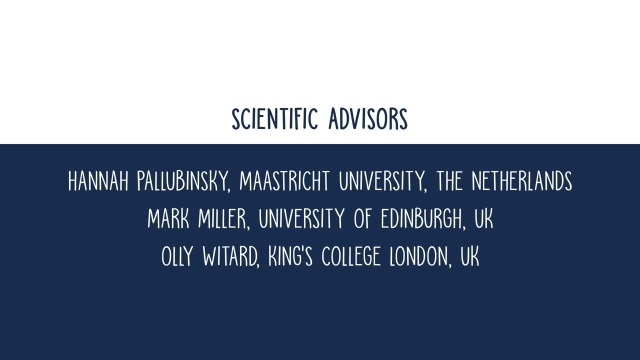 and how we can prevent it, And physiologists are playing a key role in that vital mission. For more UN videos, visit wwwunorg.